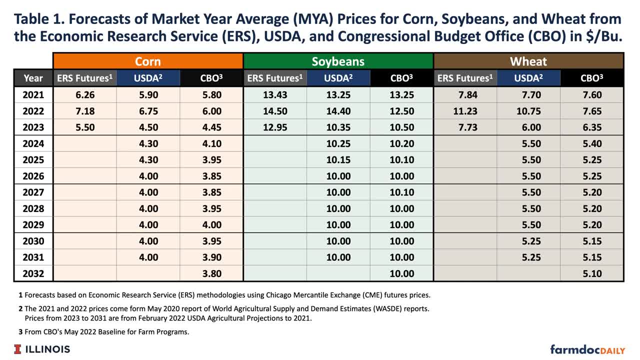 and wheat prices are much higher than those long-run averages and we have three forecasts of those prices. One is the economic research service methodology, using futures prices. USDA released their long-run prices in February and in May CBO released their long-run scores. 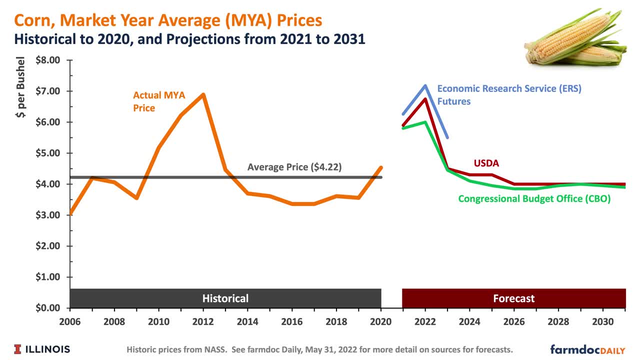 If you look at corn, the 2021 price and 2022 price are well above that $4.22 average. For example, in 2022, ERS futures methodologies forecast a $7.18 price, USDA $6.75,, CBO $6.00.. As we get to the end of the year. we're going to look at the US market. We're going to look at the US market. We're going to look at the US market And we're going to look at the US market. 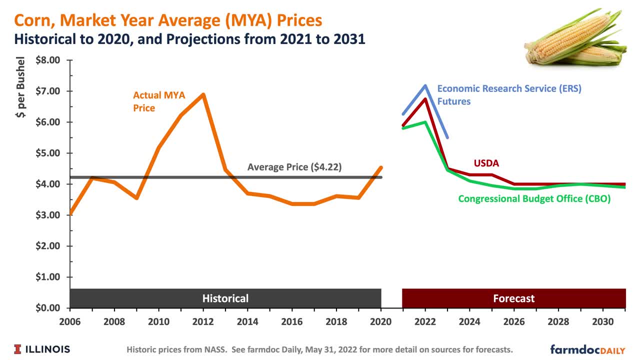 And we're going to look at the US market And we're going to look at the US market Further into the future. both USDA and CBO suggest those prices are coming down: $4 for USDA forecast and below that for the CBO forecast. 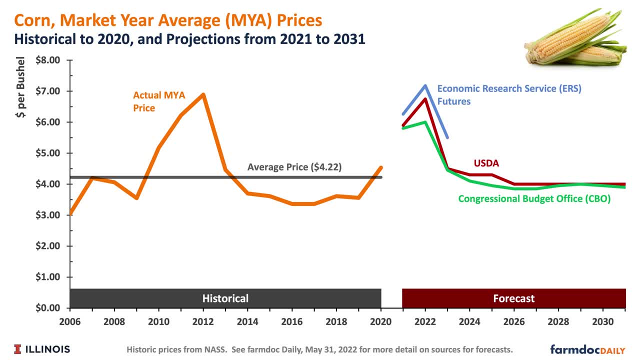 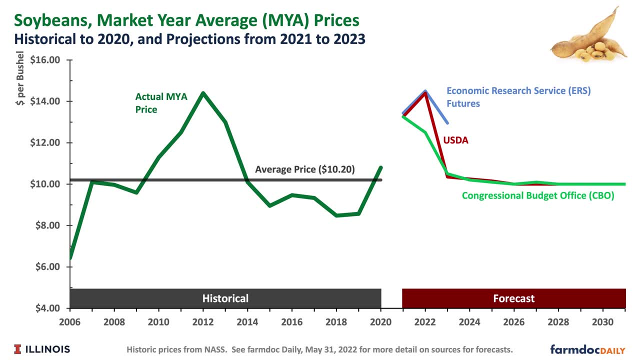 Both of those forecasts are suggesting that the current high prices are transitory. Same with soybeans. Soybeans has averaged $10.20 between 2006 and 2020.. In 2022, USDA is forecasting that price at $14.40.. 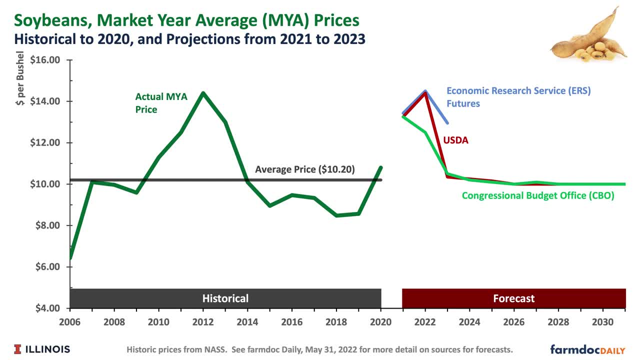 The ERS futures price is at $14.50, just a bit above the USDA forecast, And CBO is at $12.50, just a little bit below Both the USDA and CBO. have those prices again, soybean prices again coming down and reaching $10.. 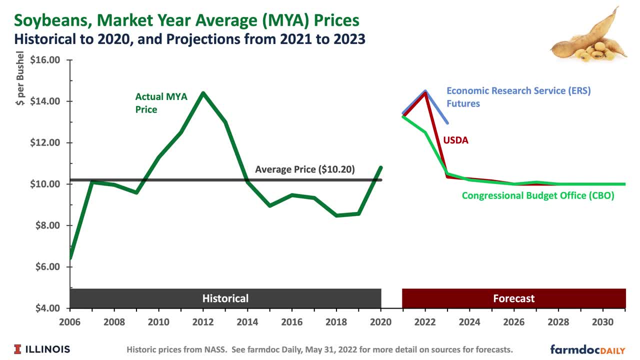 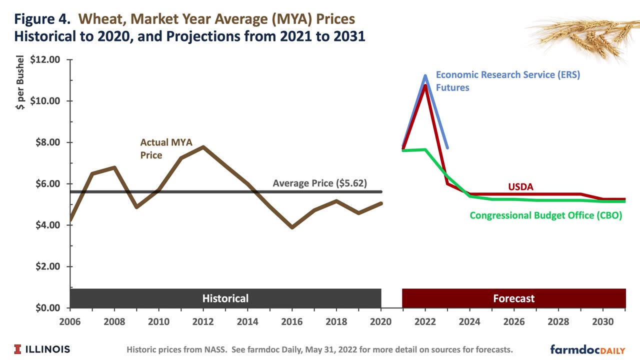 Just slightly below that average price from $10.20.. Again, Again, for soybeans. long-run forecasts are suggesting that our high prices are transitory and we will come back down. Same way for wheat: Average price from 2006 to 2020 was $5.62.. 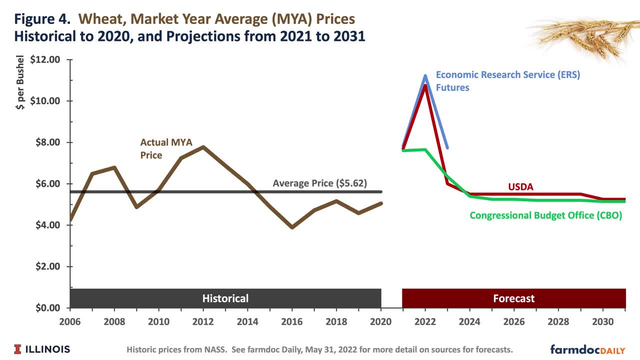 We're well above that, above $10.. Actually, $11.23 according to the ERS futures price for 2022.. $10.75 for USDA for 2022.. Again, those prices come back. USDA has that coming down to $5.25 in out years.